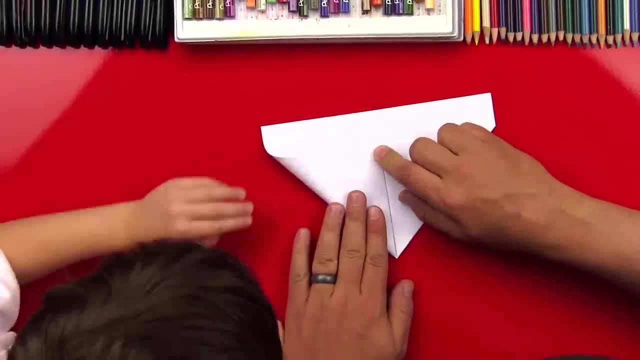 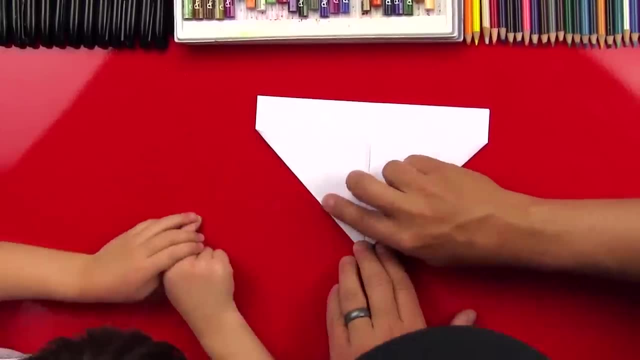 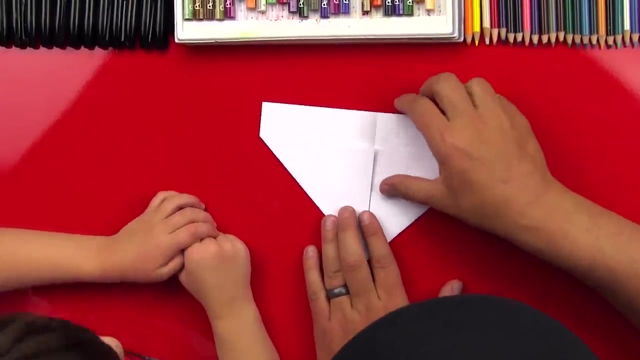 same on this side. Fold this edge to the middle also. There you go, Crease it, Boom, Good, All right, okay, Now we're going to take this edge and we're going to fold this edge to the middle Up here and we're going to fold it along this edge. Here we go, We're going to fold it all the. 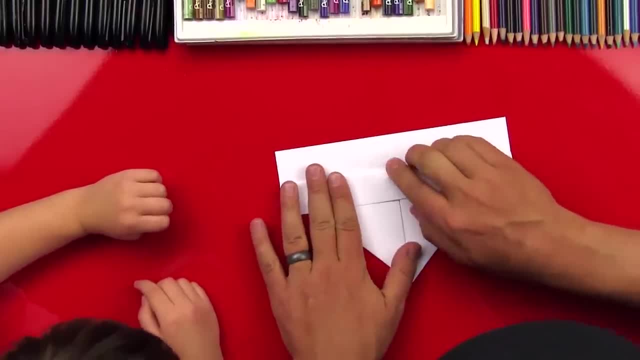 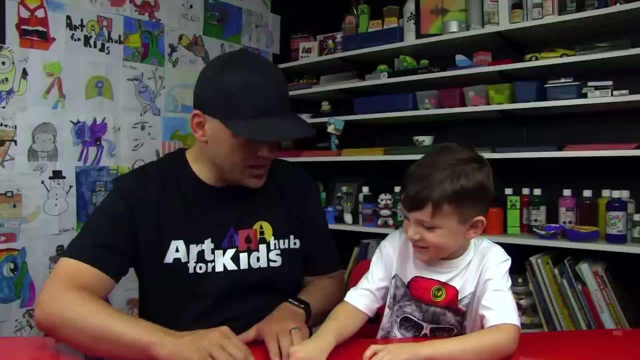 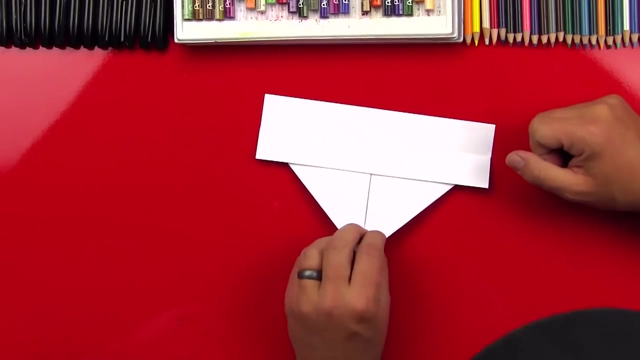 way down like this, and then fold it flat. Can you crease that side? Crease it right over here? Yeah, Good job, You got to make noises when you crease. Yeah, there you go. Use your muscles. Okay, now we're going to flip it over. and now we're going to fold. We're going to fold this. 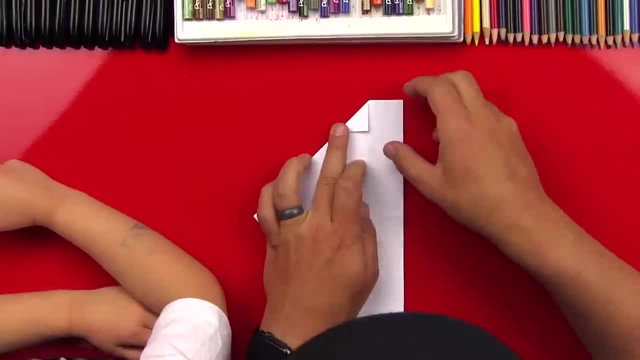 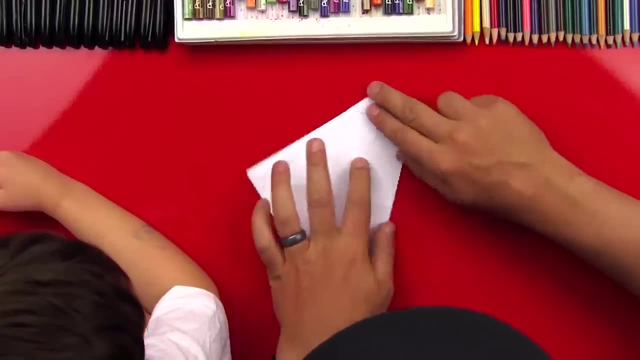 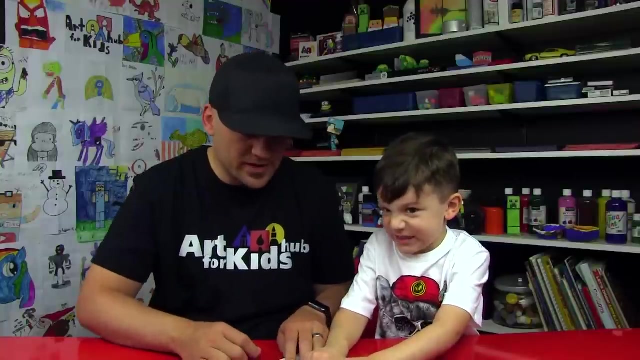 corner down like this Right here, And then we're going to fold this corner like this. Is that cool? Yeah, Kind of like we're making a little airplane. We got a little triangle right there, So let's do it on this side too. Can you fold this over, Fold that down, Crease that, Crease that. Oh, muscles. 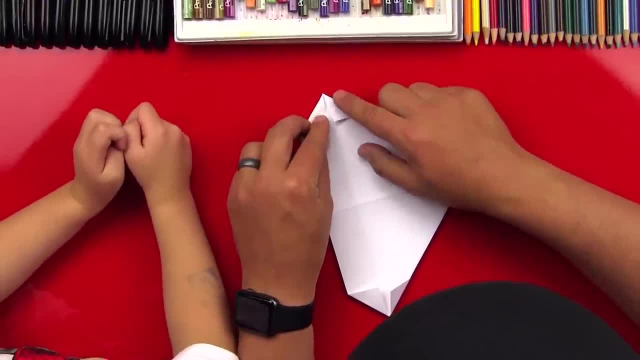 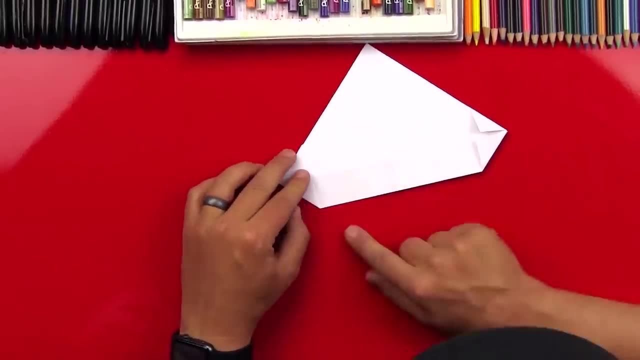 Then we're going to fold the same thing. We're going to repeat the step where we fold this corner like that Isn't that cool? Yeah, Okay, turn it like this: We're going to fold this edge up so that it matches on the other side. 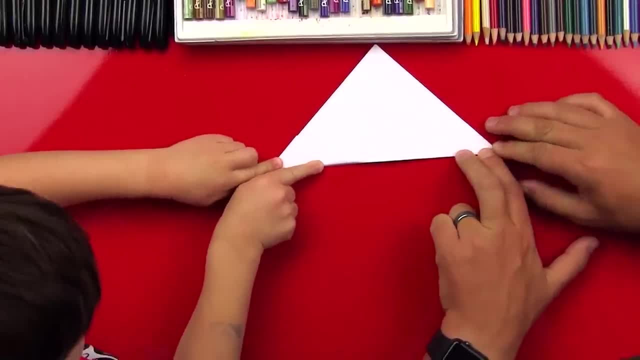 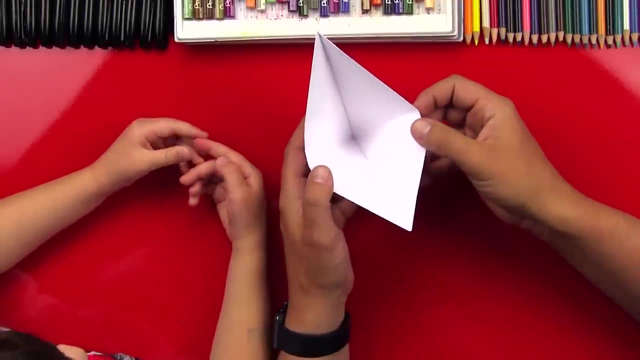 We'll fold right there. Okay, do it. Yeah, Keep going. Okay, now we're going to pick up our model and we're going to open up. Look at that, It's like a little pocket. We're going to open it up. 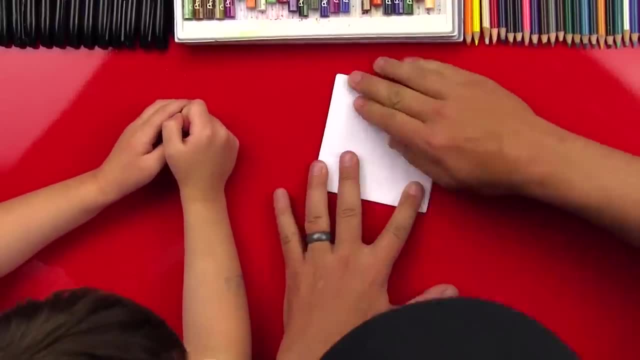 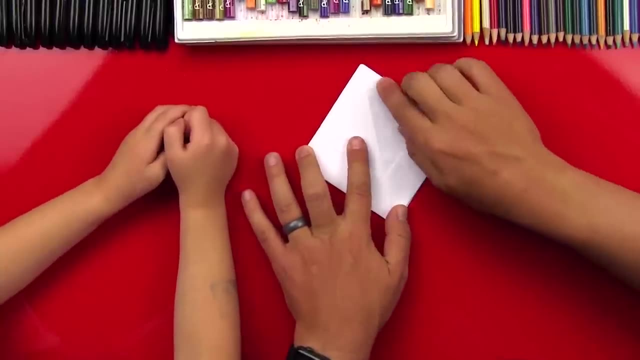 and then fold it down so it makes a triangle. Well, not a triangle. What is that shape? Diamond, Diamond or a square? There we go, That's the right shape. Then we're going to cut it, Crease these sides down like this: Okay, now we're going to take this corner. We're going to 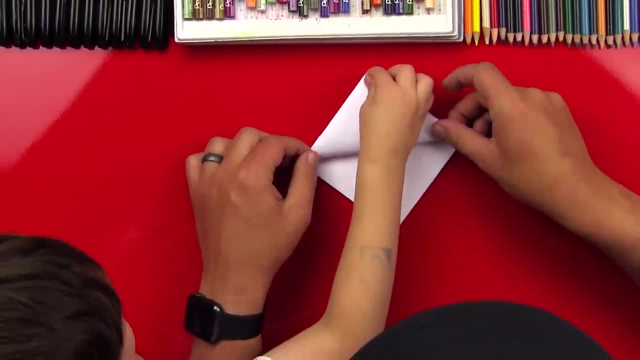 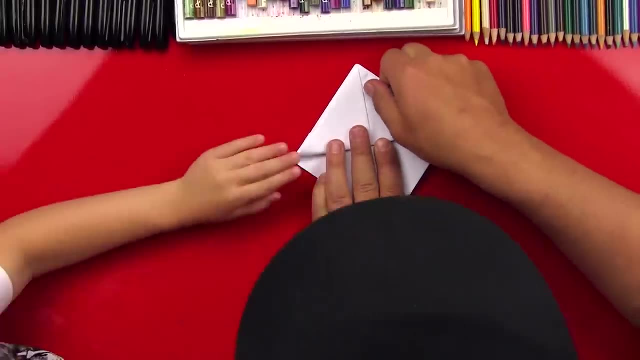 fold it up to that corner, Good job. Fold it all the way up there, and then we got to press it down here. Let's pull it up just a little further. There we go, Crease it, Good job, Good job. 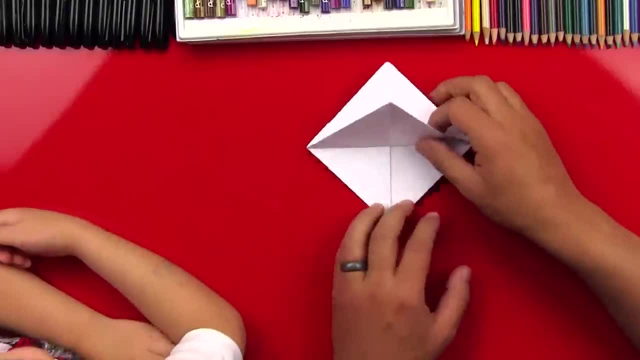 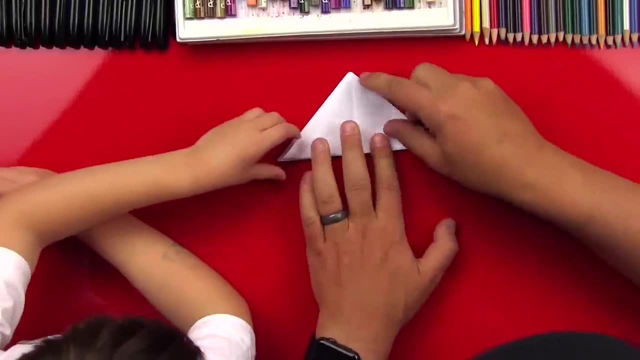 All the way, Muscles, Muscles. Then we're going to flip it over and we're going to repeat that same step Over here And put that over there, Yeah, And we fold that down like that. So now we got a small 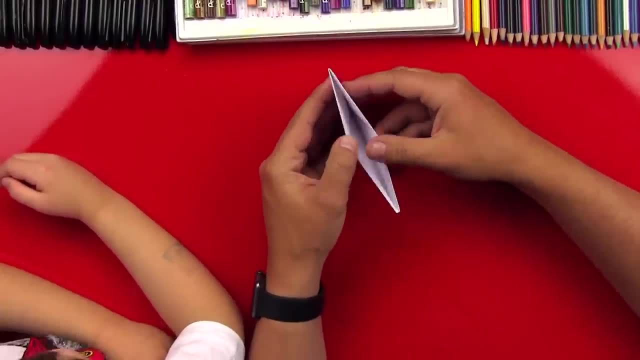 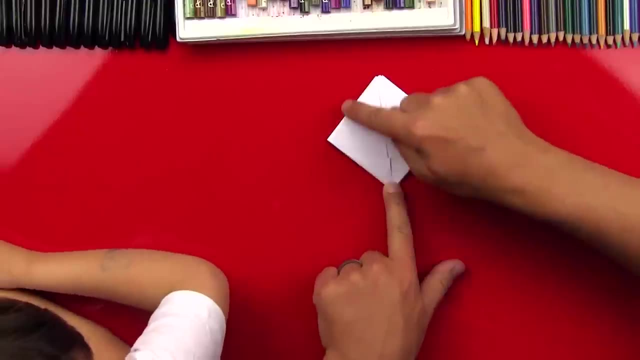 triangle and we're going to do the same thing. We're going to pick it up and we're going to open it like a little pocket. Is that cool? Yeah, And then we're going to flatten it down so it makes another. What is that Diamond? Yeah, another diamond, Isn't that awesome? Yeah, Okay, we're. 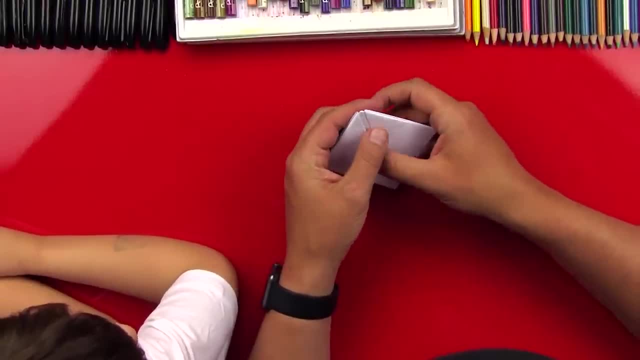 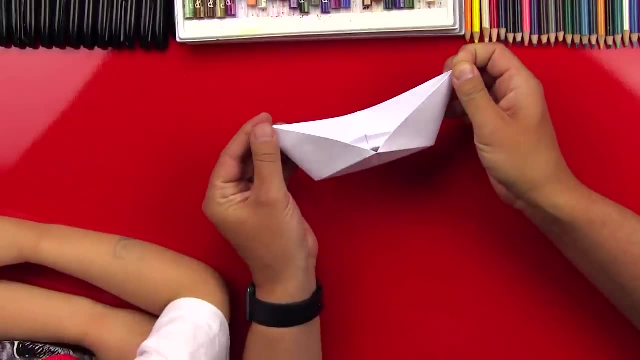 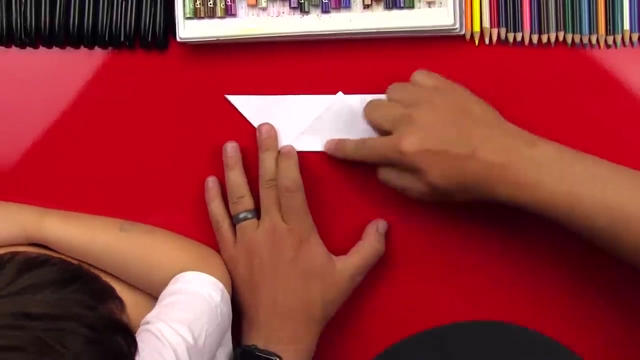 almost done. See, up here at the top, we've got these two little corners and we can pinch the corners, Yeah, And then open it up. Is that awesome? Yeah, And we just keep opening it up until it lays flat. That was like magic, wasn't it? Yeah, Look at that. Press really tight, Press that down. 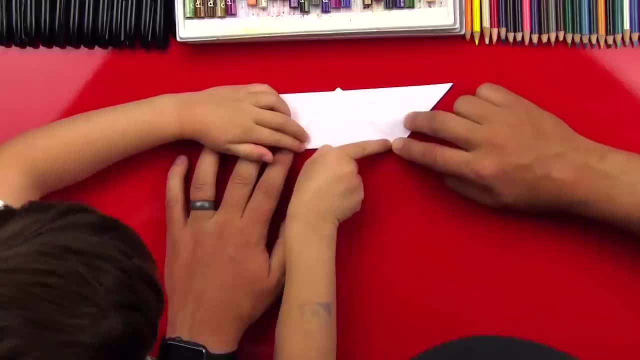 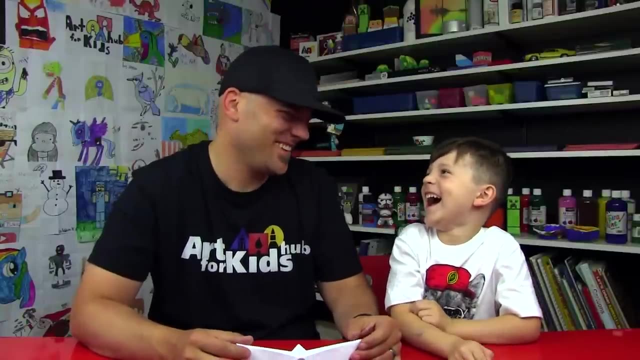 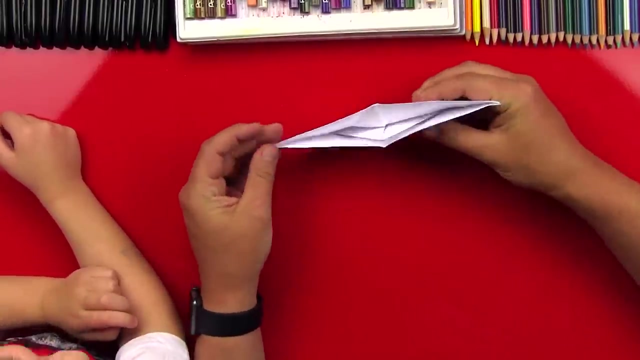 Crease it. Good, All the way across. You're not pressing hard, You're just pretending. Look at this, It's a little boat, Isn't that cool? Yeah. And then we got the little sail inside there. That's awesome, huh, Yeah, Give me five. You did a good job, And we have a bowl over here full of. 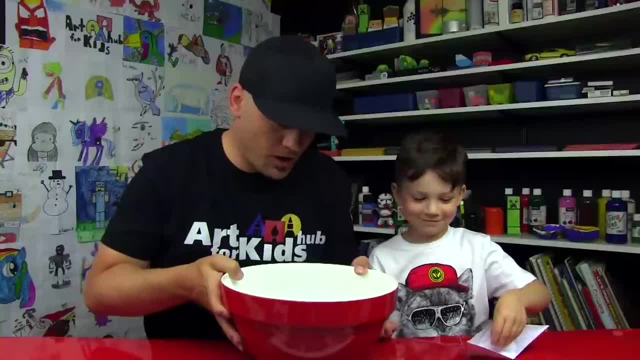 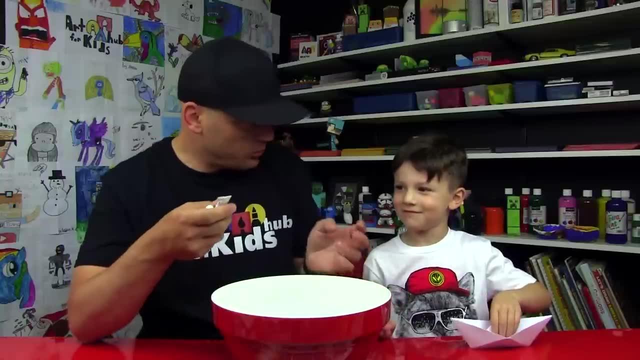 water. Should we see if it floats? Yeah, Okay, dude, Here's our bowl of water. We're going to test it and see if it floats. And you know we should use a different kind of paper. We could use wax paper that's waterproof because it's not going to float very long, And we have these. 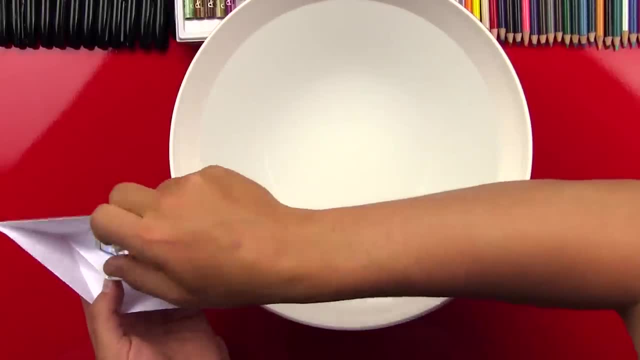 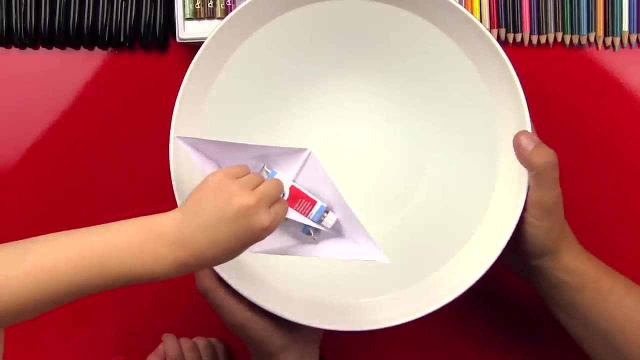 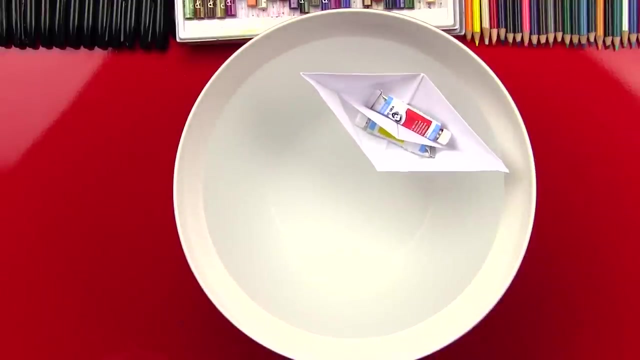 little paints we're going to put inside So that'll help it stay upright, Otherwise it'll just tip over. Okay, you put it in there, Hold it by the sail, And we're going to test it And we're going to drop it in. Oh, that's awesome, Good job, Give me five. Look at that, It's floating, It's. 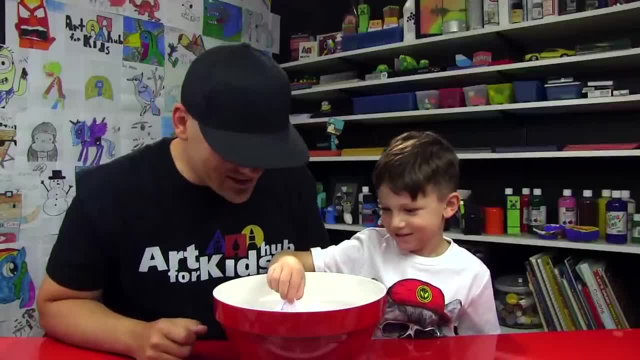 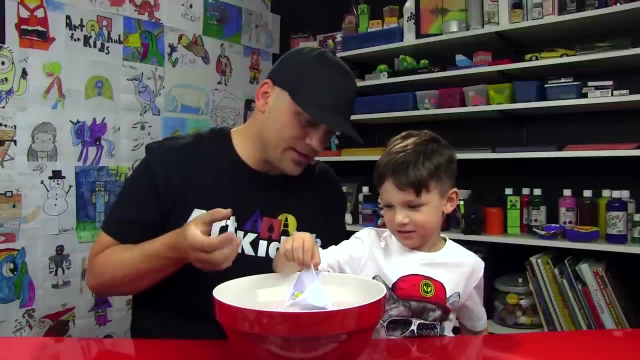 only going to float for a little bit until it gets soggy, Sinking. Oh, it's sinking. If you guys use different paper, it won't sink, It won't get soggy, It won't float to the bottom, It won't sink to. 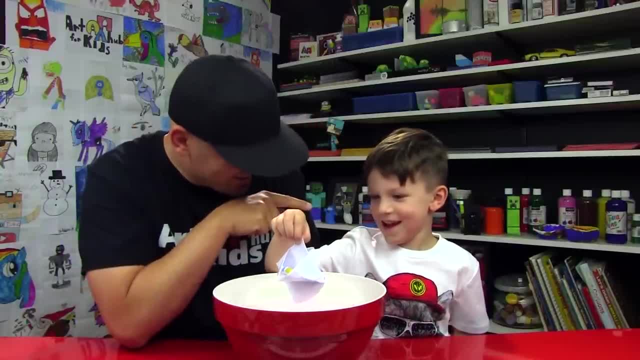 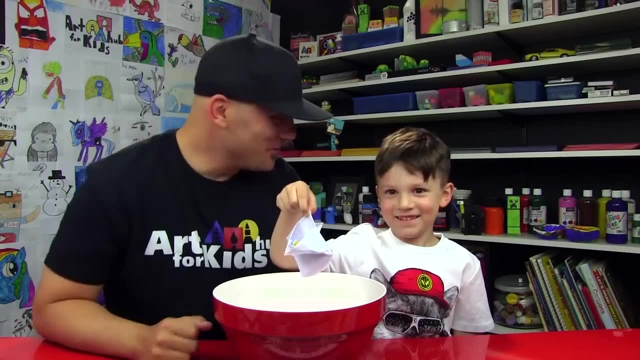 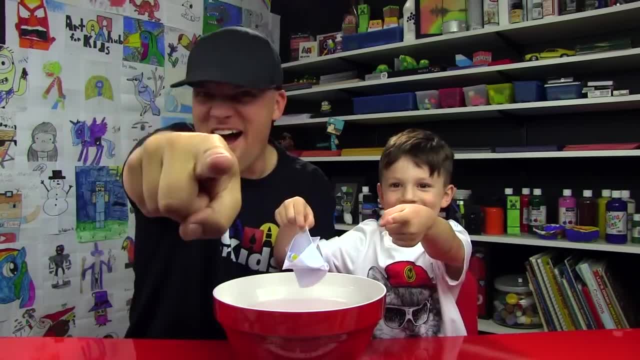 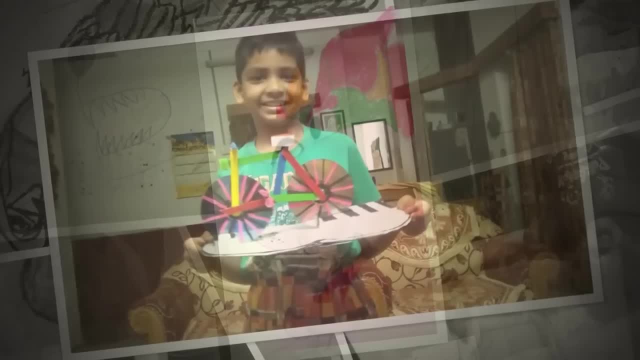 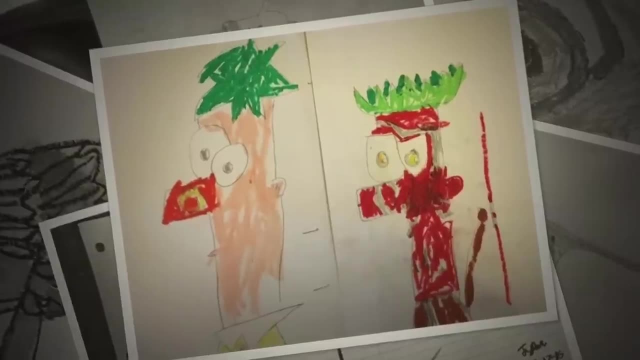 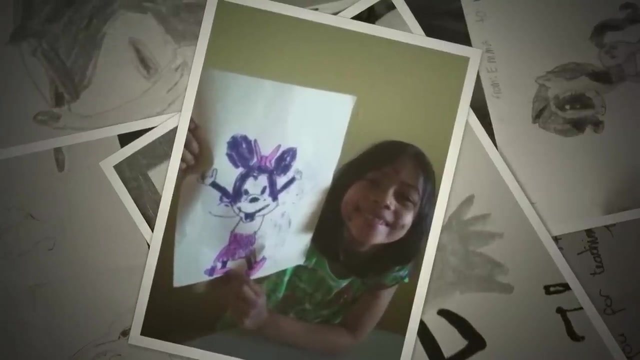 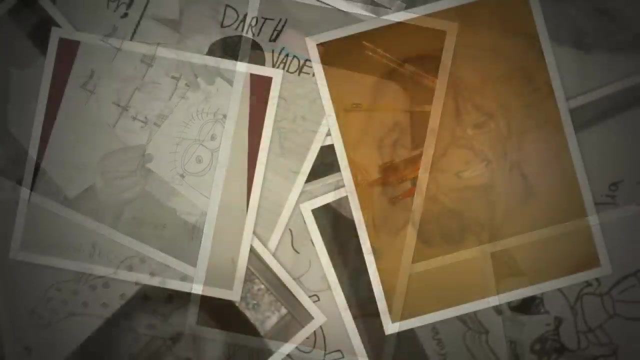 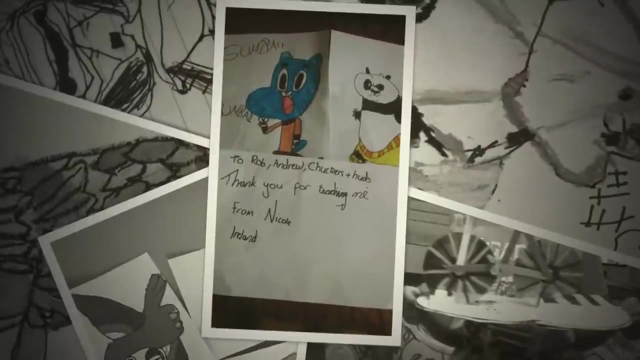 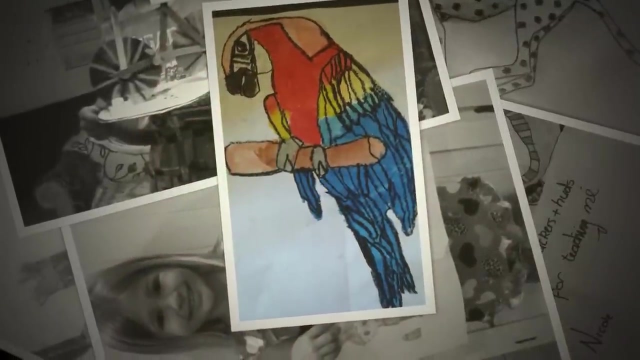 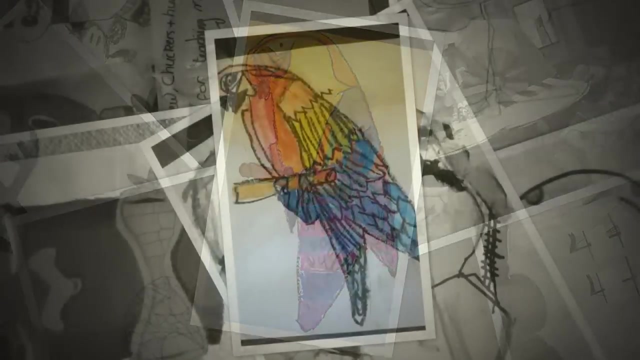 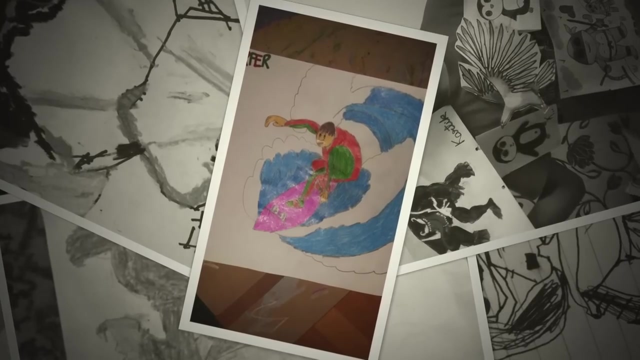 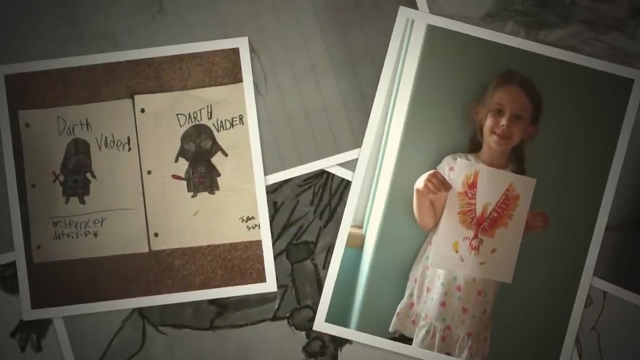 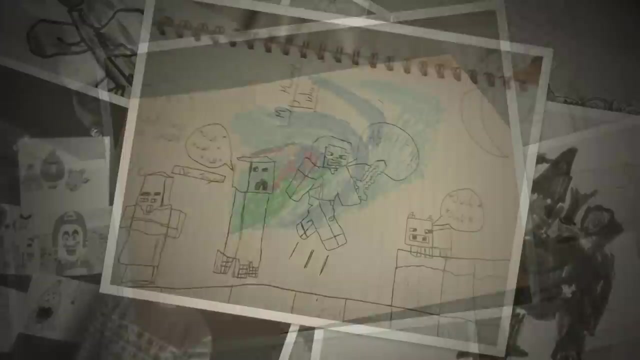 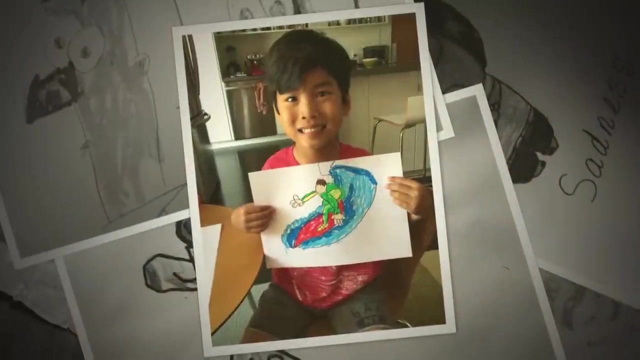 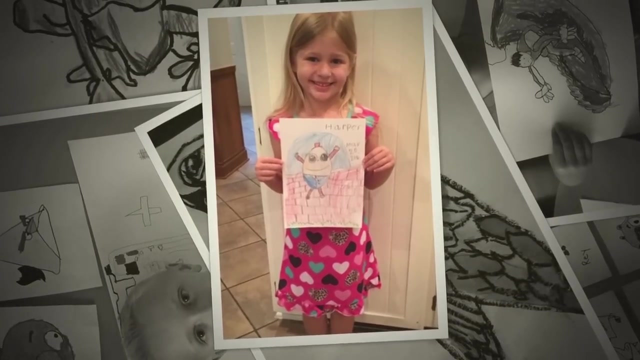 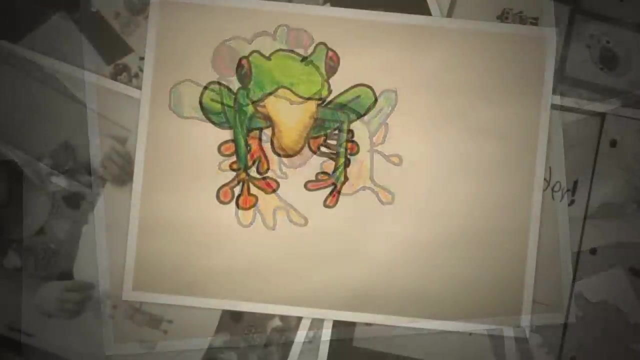 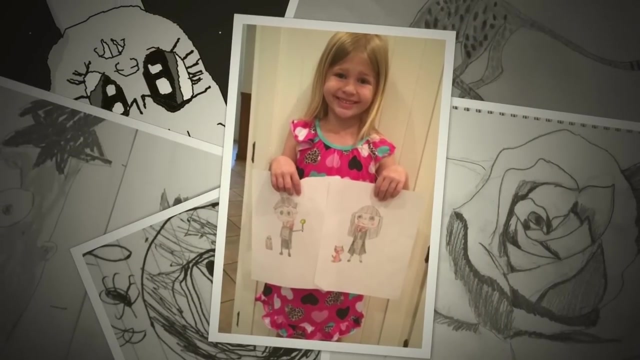 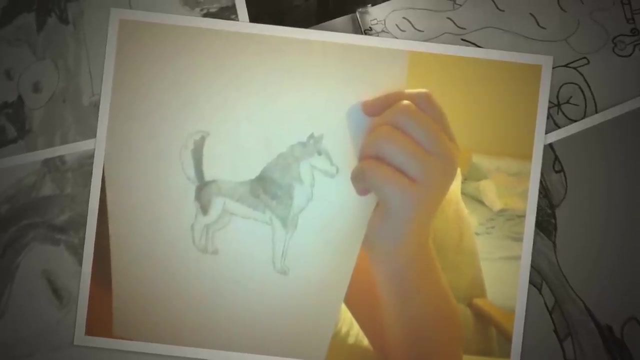 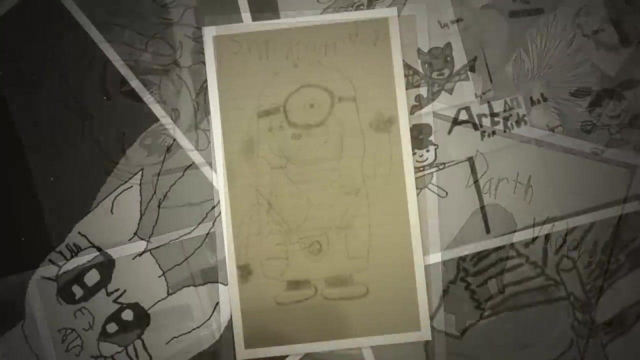 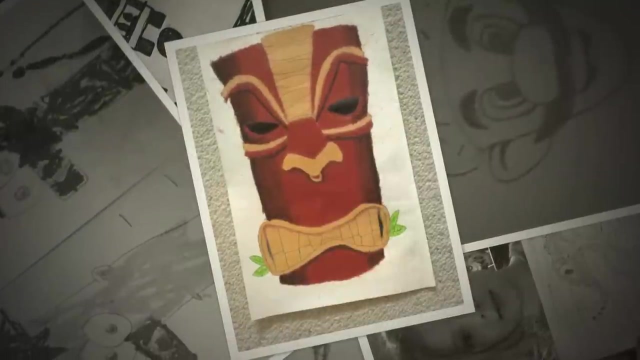 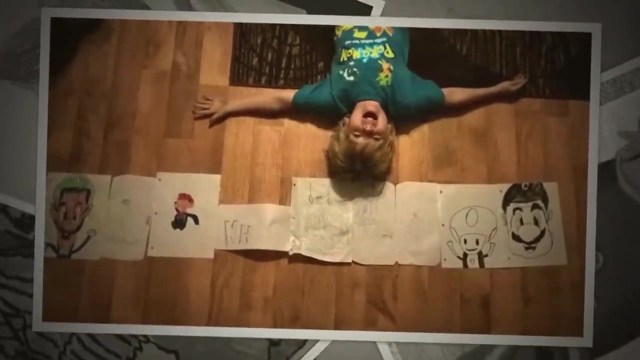 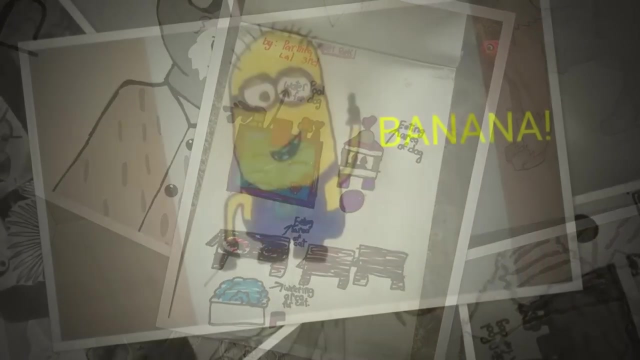 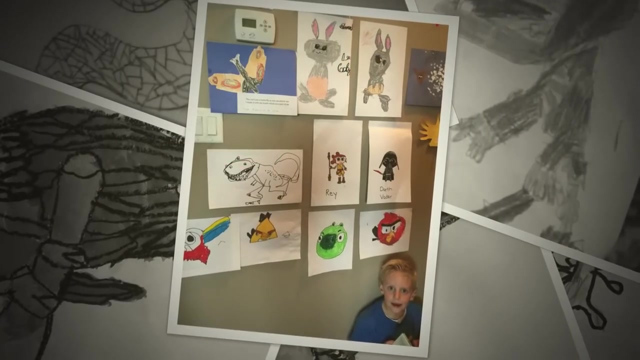 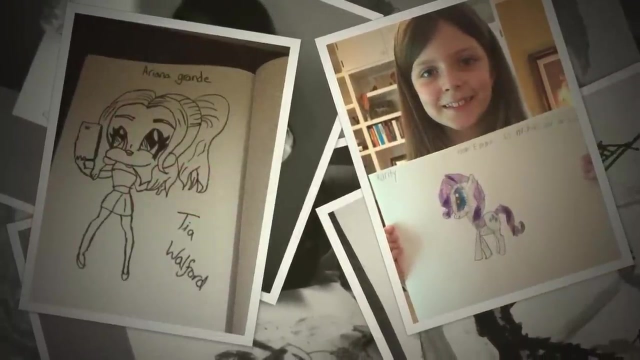 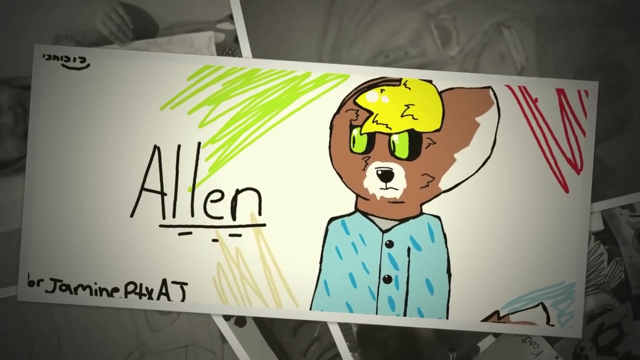 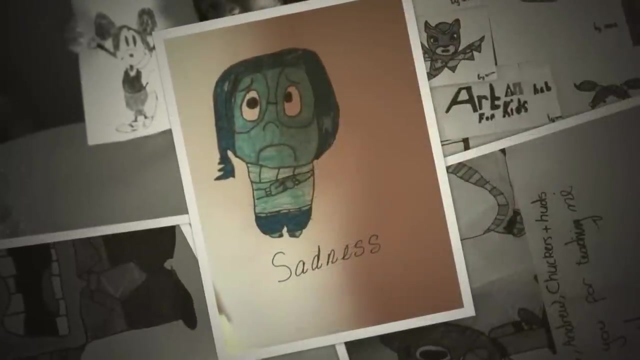 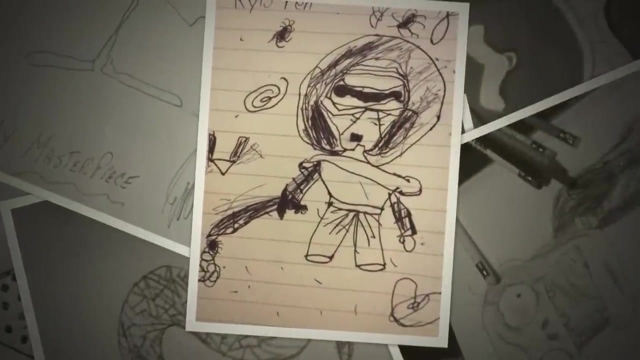 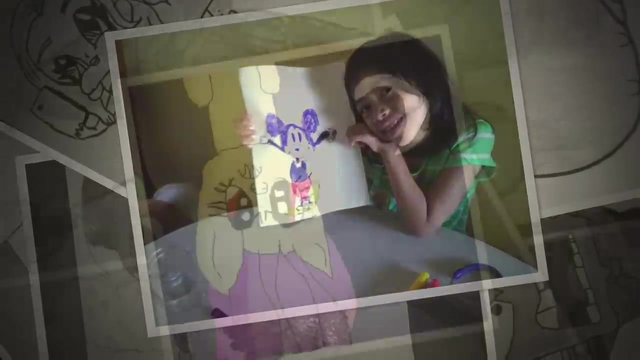 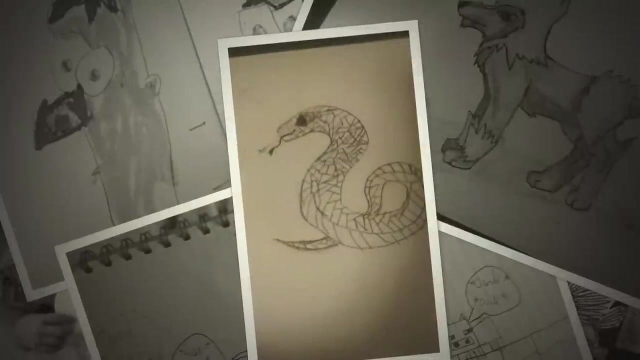 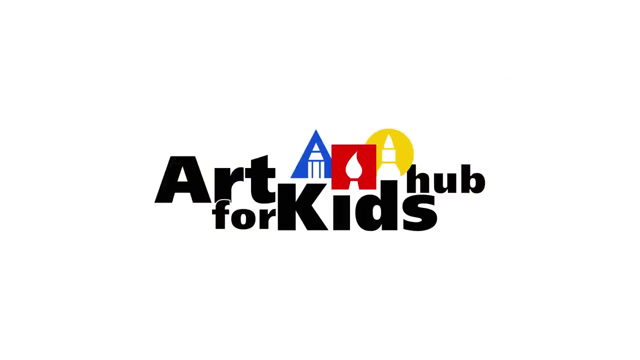